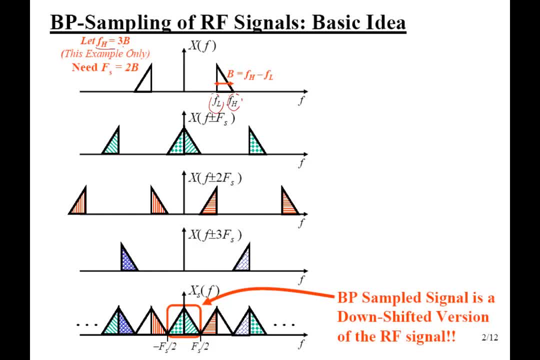 FH is the higher frequency and FH is equal to 3 times the bandwidth Right And FS. let's say we sample this particular passband signal at FS is equal to 2B. Now, as per Nyquist criteria, we have to sample it at least greater than 6 times B. But here we are saying that we 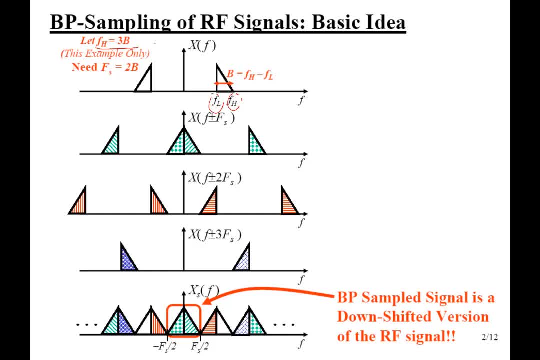 are not following Nyquist criteria and we sample it at a sampling rate of 2 times B. So if we sample at 2 times B, you see we will definitely get multiple copies, because whenever you perform sampling you will get multiple copies at integral multiples of the sampling. 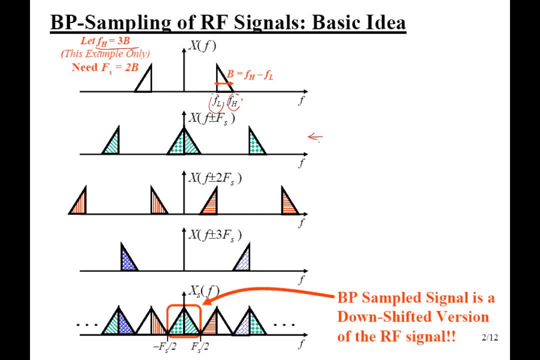 frequency. So for example- first copy that you will obtain at plus minus fs, this is the second copy that you will obtain at plus minus 2fs, this is at plus minus 3fs, and so on, and if you add them all point by point, then you 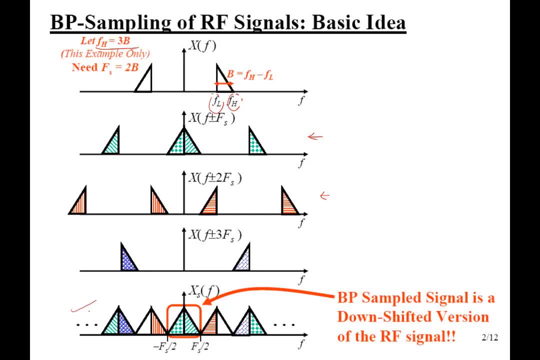 will get this particular result and in this result you can see that the actual spectrum of that pass band signal is recovered in the form of a low pass equivalent signal. these two copies- the right side copy and the left side copy, both are now located at the base band. so in this way, without following, 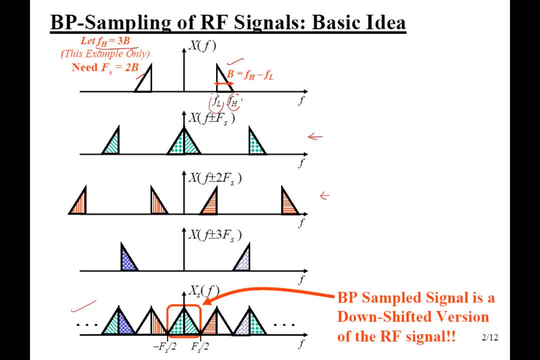 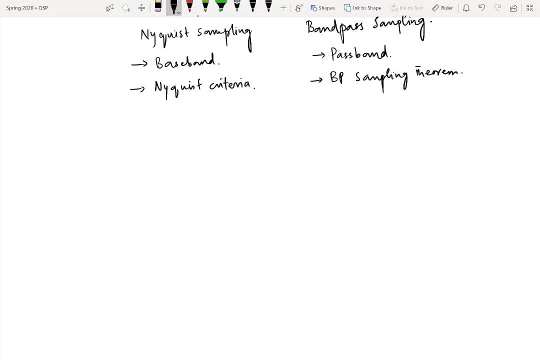 the nyquist criteria, we sample the pass band signal at a lower sampling rate still, we are able to avoid aliasing. so now we can formulate two different cases, such that the higher frequency fh is equal to k times b, where k is an integer or unknown integer, and in the first case we can further have two cases. if k is an integer, it can be odd. 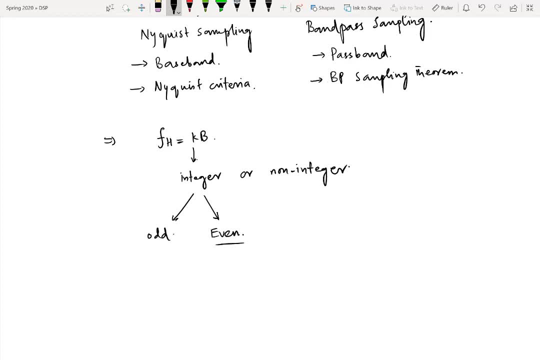 and it can be. even so. it means we will first find out the bandwidth of the pass band signal and then the higher frequency of that pass band signal, and we see that. what is the situation of this number k? if that is an integer, we are into the first case. if it is a non-integer, then we are. 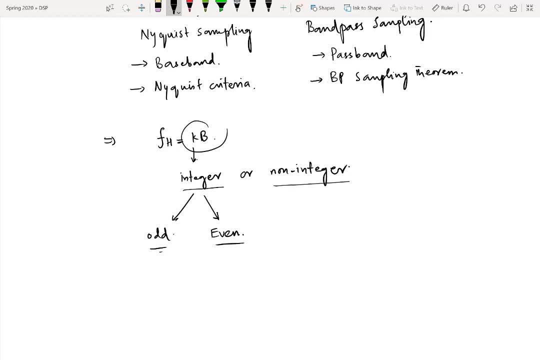 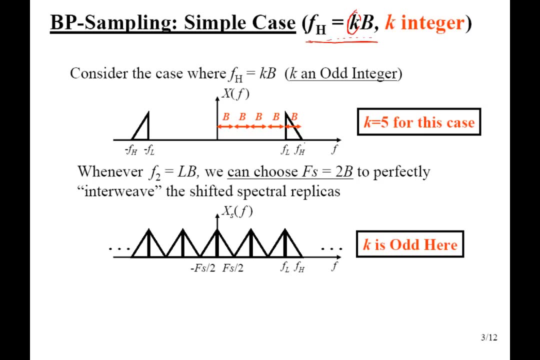 into the second case. and being an integer, it can be odd, or even so. if that k is an odd integer, what will happen? you see, this is an example where fh is now five times b, so k is equal to five, in this particular case, five times the bandwidth. again, we can choose. 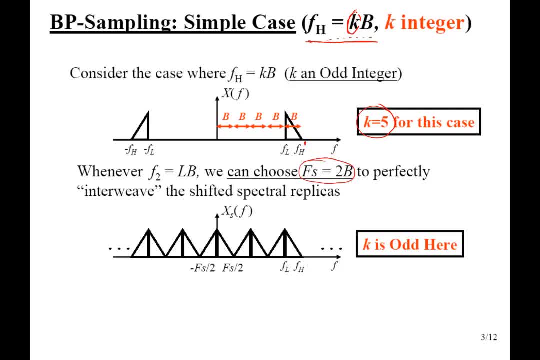 fs is equal to 2b, two times the maximum bandwidth. we select this criteria for the sampling and if we sample at this sampling rate, then, by using the same technique just discussed earlier, you can see that the actual copies of the pass band signal are now located at the 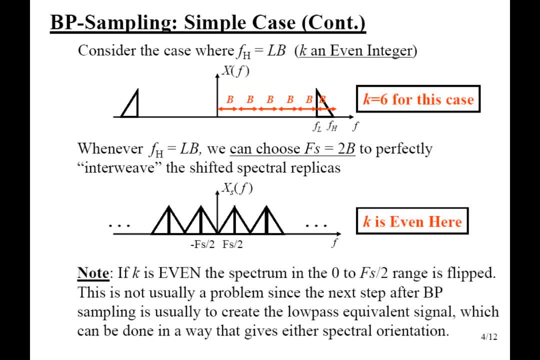 base band in the form of a low pass equivalent. and if k is an even integer, like for for this example, if k is equal to six, then fh is equal to here. fh is equal to six times b. so for this particular case now, if you again sample fs at fs is equal to 2b, this spectrum, then you will see. 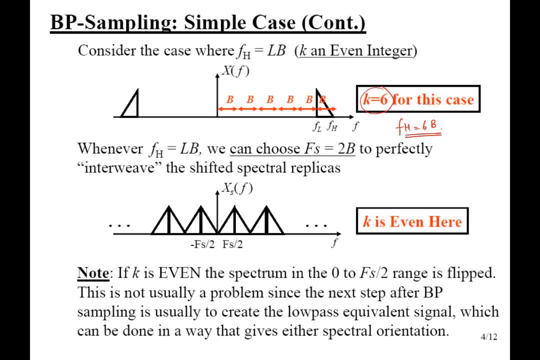 by following the same procedure, you will see that now you will get the the same two copies of the pass band signal at base band. but the difference is that these two copies are flipped. the right-sided copy has gone to the left and the left-sided copy has gone to the right. but that flipping is not a big problem. 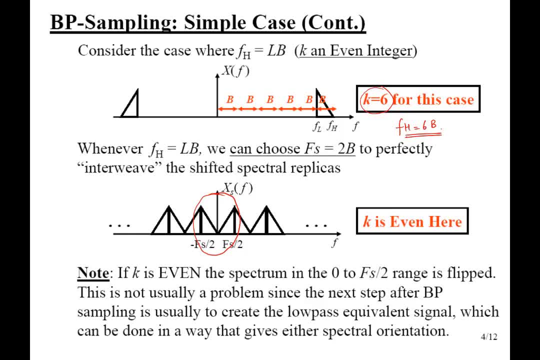 because in in any case, we are going to formulate a low pass equivalent model, and for low pass equivalent, it doesn't matter that either the copy is located on the left or it is located on the right. simply we need to low pass filter it and then we can adjust the content of the right-sided. 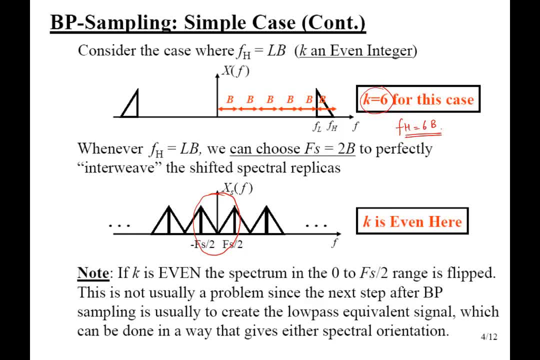 and left-sided copies. so it means that when k is an integer, either it is even or it is odd. it is not a problem. we do not encounter any problem of aliasing if we sample at fs is equal to 2b. but remember this is not always true that k is an integer. in most of the cases k is not an integer. therefore this: 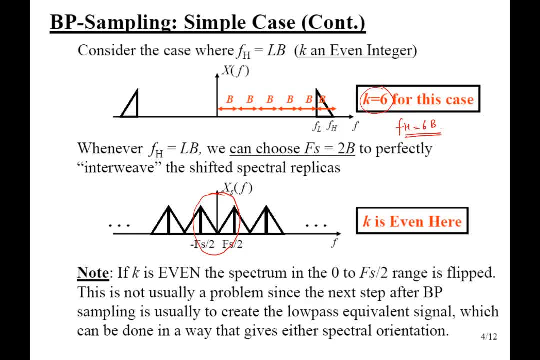 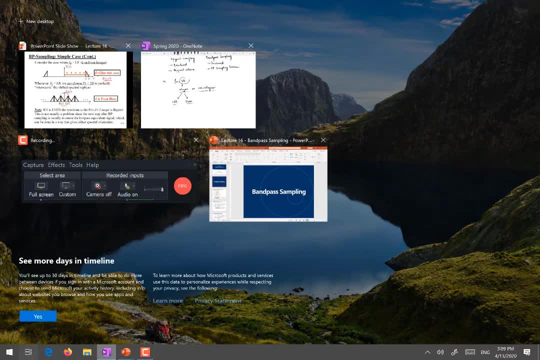 approach cannot be followed in general. we need to formulate a generalized mechanism to find out the pass band signal, at which sampling rate we need to sample the pass band signal so as to avoid the aliasing right. so for this we consider a generic model and try to find out the criteria for. 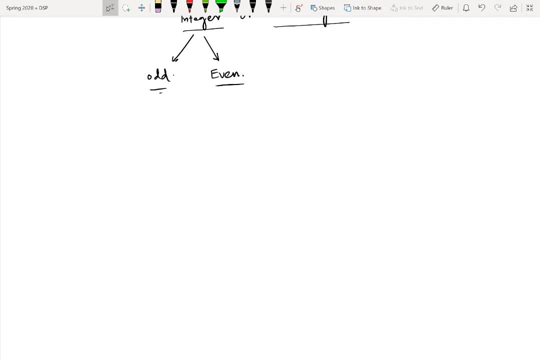 sampling the pass band signals. and to have that criteria. let's suppose there is a pass band signal and to have this criteria: let's say there is a pass band signal whose spectrum is like this, with the bandwidth of capital b, this point is f l, this point is f h, and. 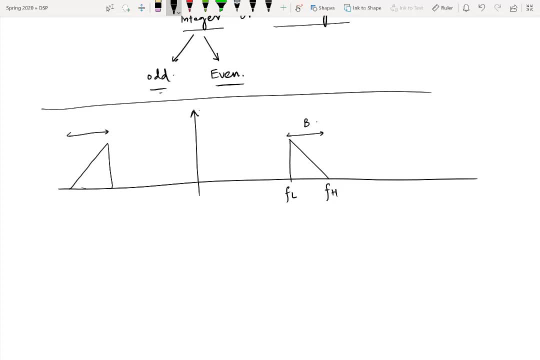 similarly same thing on the right side and just to see the difference, we can consider the opposite copies. it is minus f h and it is minus f l. right now, let us consider any arbitrary integral multiple of the sampling frequency. so let's consider any arbitrary integral multiple of the sampling frequency. 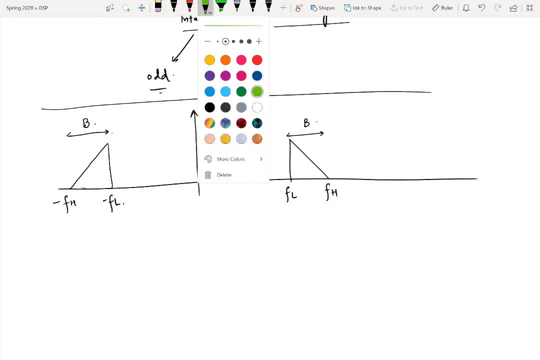 let's say we talk about the integral multiple of the sampling frequency in the form of k minus one times fs. so at this sampling frequency, the right-sided copy, which is this one? the right-sided copy? let's assume that it comes somewhere over here, and the right-sided copy definitely is on. 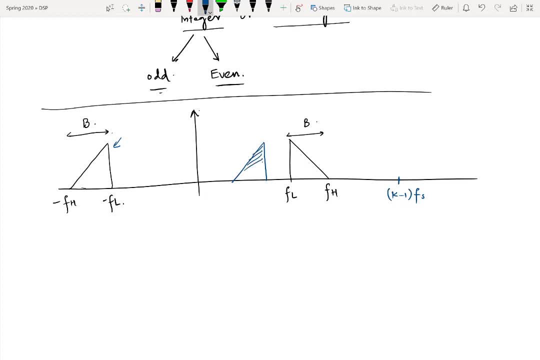 the right, which i am not going to plot. so this is your left-sided copy, corresponding to k minus one fs right. similarly, let's consider another frequency, which is k fs, the next two k minus one. so for this k fs, again the left-sided copy. let's assume that it comes over here. 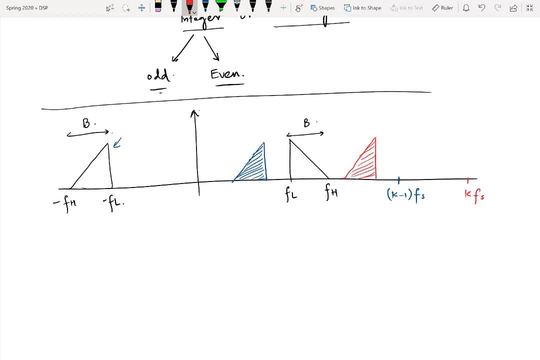 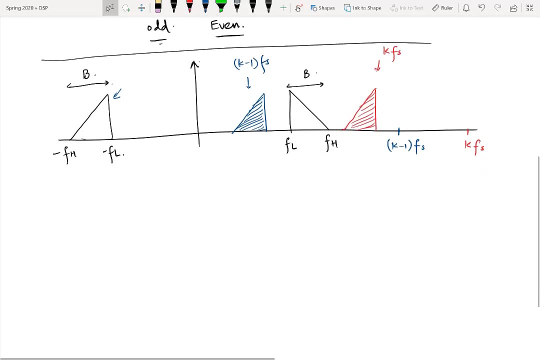 and again, i am not plotting the right-sided copy, it will be somewhere on the right. so these are the two copies, this copy corresponding to k minus one fs, and this copy is corresponding to kch общ madness of k times fs. now we have to formulate some labeling in order to find out. 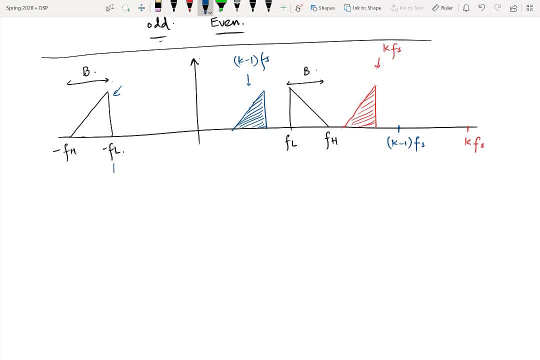 the condition. first of all, let's let us see that the range from this point to this point, what is this range? because from this point, from origin to fn, it is fn and same on the other side, so you can say that it is two times f? l right. this is the first point. and secondly, 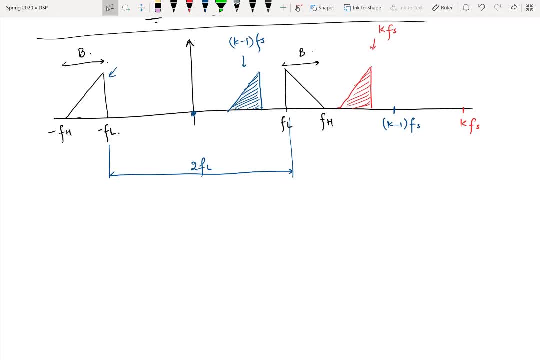 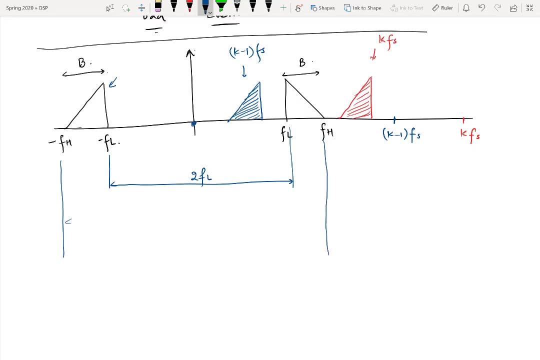 What about FH? For FH, you should observe that this particular point and this particular point, If you see this range, it comes out to be 2FH. Okay, now you see, this point is K minus 1FS. So the distance from here to here, this is K minus 1FS. 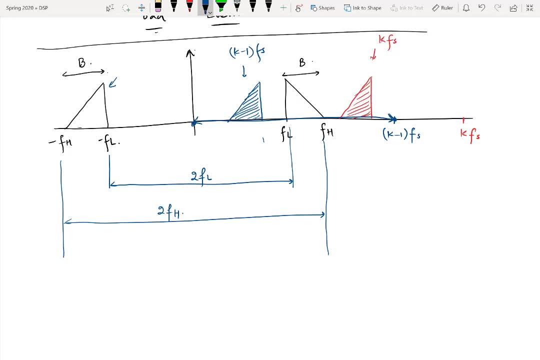 Right. But if I subtract this distance, this range, which is what, This is basically equal to FL, because it is corresponding to this much, because this copy is actually shifted at the at K minus times FS. So it means this range is equal to FL, Right. 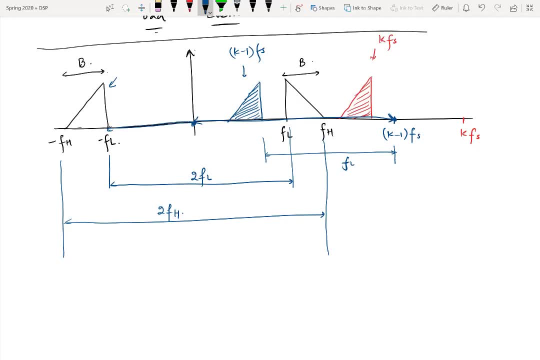 So if I take this FL over here at this point and I mark the range starting from here to here, so you see what should be this range, This must be equal to FS into K minus 1, because from this point to this point it is K minus 1FS plus FL. 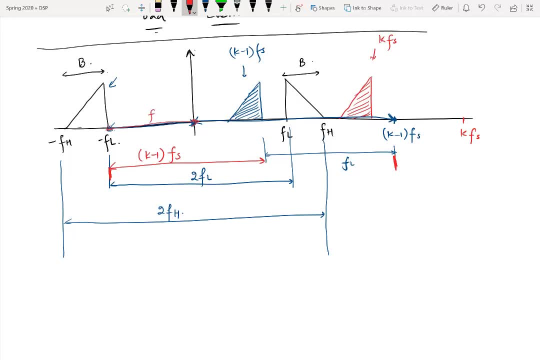 Right And this distance is also FL And this distance is K, K minus 1 into FS. So I have just swapped the two variables. I have taken FL towards the left and FK minus 1FS towards the right. So in this formation it is K minus 1FS. 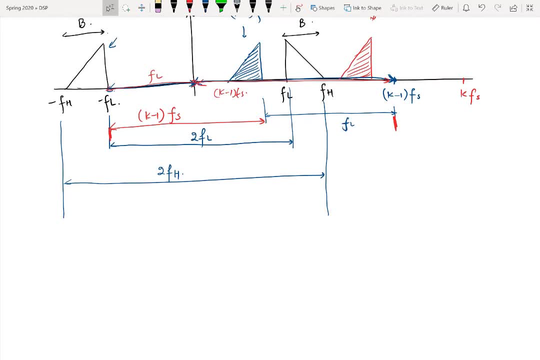 Similarly, by using the same approach, you can also label here K times FS. So if I start from FH and I go until the lower end of this point, So what about this range? This range will be K times FS, by using the same approach as I have already told you about K minus 1FS. 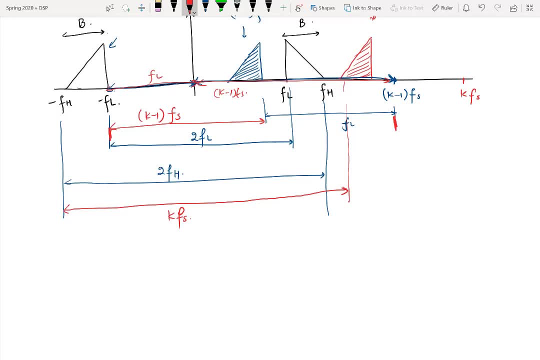 Right, So these are some variables that need to be labeled. Now, if I want to avoid aliasing, it means I will want that this point and this point they must be distant from each other. They must be distant from each other. 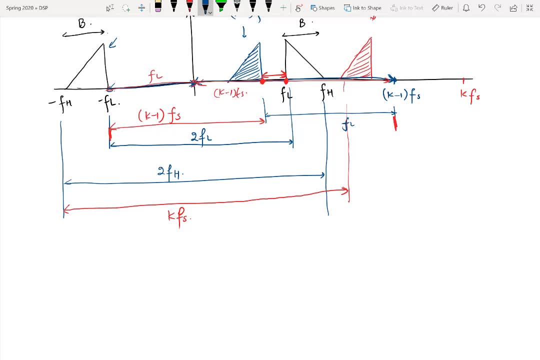 It means the first condition. The second condition that I have is that K minus 1FS must be less than or equal to 2 times FL, because the first red dot is corresponding to K minus 1FS and the second red dot is corresponding to 2 times FL. 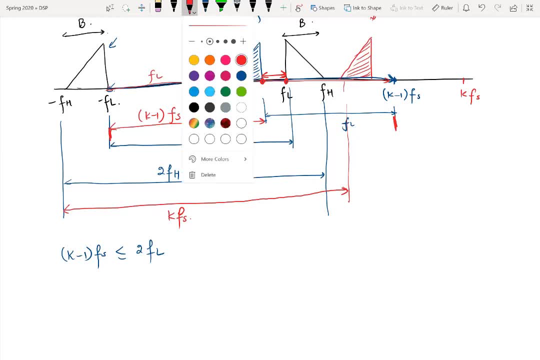 OK, so now, what about the second condition? Now I also want to avoid aliasing by keeping this point less than the second red dot. The first red dot is what It is, 2 times FH, and the second red dot is KFS. 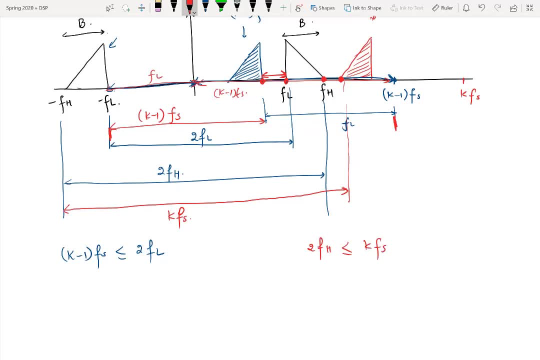 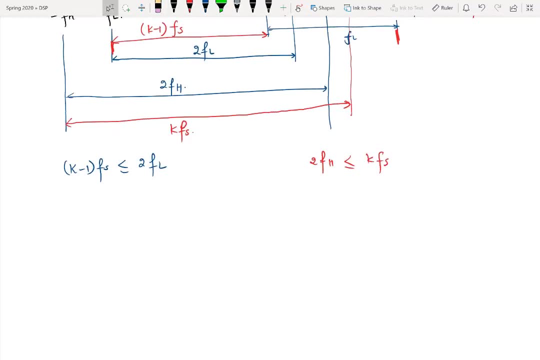 So it must be less than KFS, Right? So I have got these two inequalities. Now let us try to solve these two inequalities and try to find out some condition, And by using the fact, of course, that B is equal to FH minus FL, so that FL is equal to FH minus B. 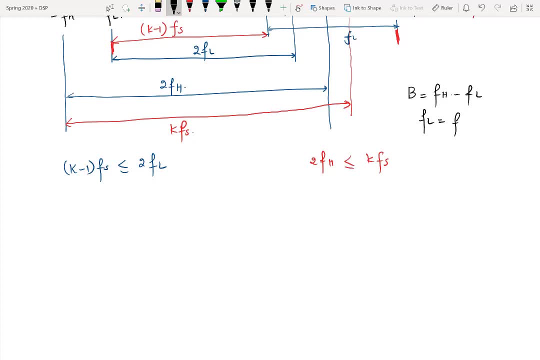 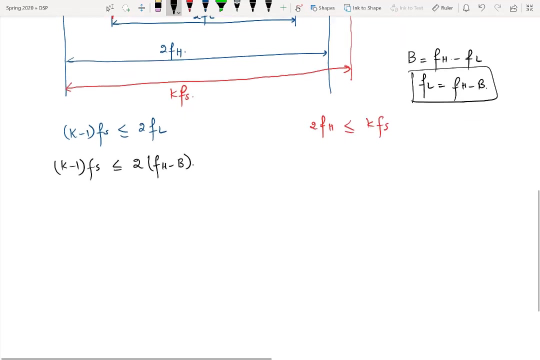 FL is equal to FH minus B. FL is equal to FH minus B. OK, so here it becomes K minus 1FS, less than or equal to 2 times FH minus B, And from this inequality we can write: 1 over FS is less than or equal to K over 2 times FH. 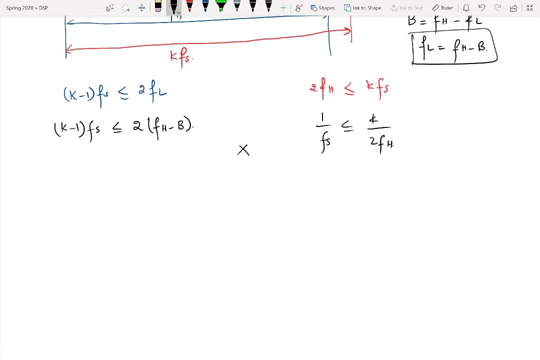 Right Now. if you just multiply these two, If you multiply these two inequalities Right, The resultant will be: Because the direction of inequality is the same. So we can directly multiply Right side with right side, And left side becomes 2K FH minus B divided by 2 times FH. 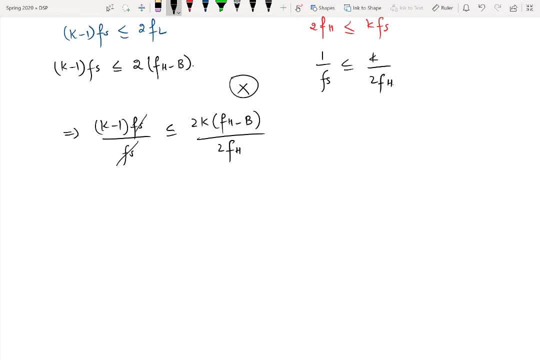 Now, if you solve this inequality, FS is cancelled out from here And on the right side it becomes 2K FH divided by 2FH, 2FH minus 2K B divided by 2FH. So here FH is cancelled out. 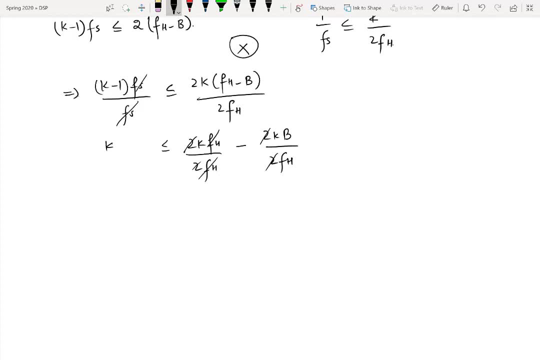 2 is cancelled out, Here 2 is cancelled out, And here we are left with K minus 1.. Further solve it to get here K as common into 1 minus B over FH. If you solve this inequality for K, you will end up with this inequality. 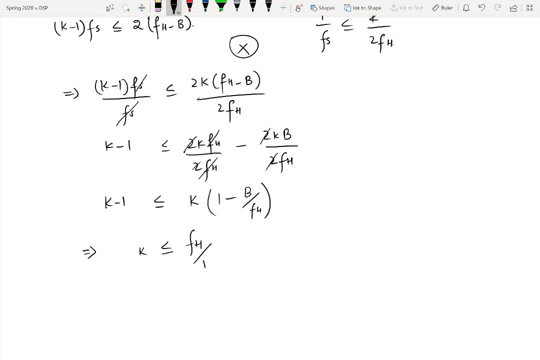 K less than or equal to FH over B Right. So less than or equal to means if you want to have, if you want to, So K less than or equal to FH over B means if you want to have an integer value of K, then what we will do. 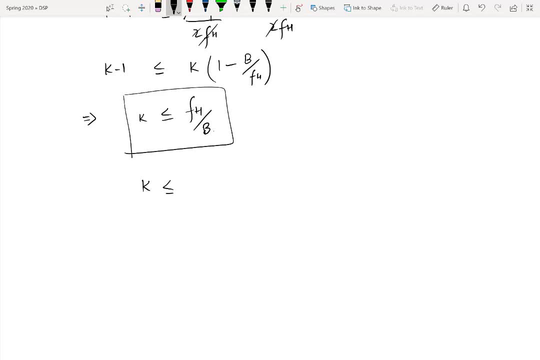 We will just floor this result, So it will be equal to FH over B. Or we can also say Now, if you want to have, if you want to find the maximum value of K, that will become of course by flooring the result. 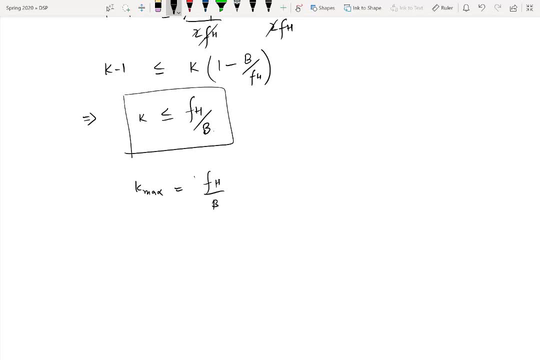 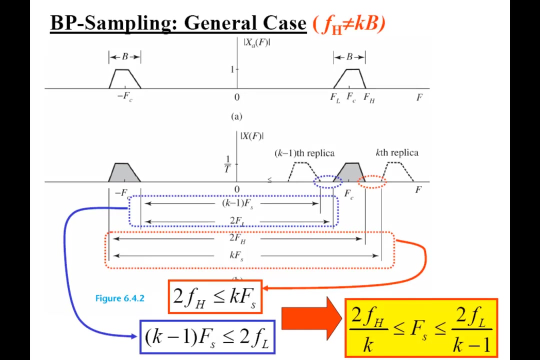 So it will be equal to FH over B floor. So that is basically the maximum value of K that you can use Right. So now we see what is happening over here. So we have actually got two conditions. The first condition is this one: 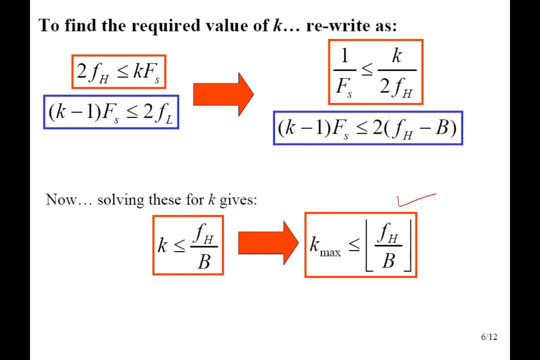 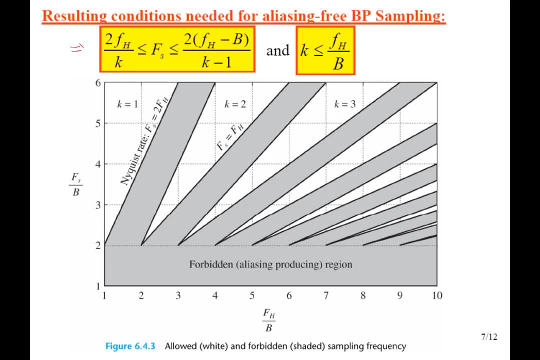 Which is K max less than or equal to FH over B. And the second condition, which is necessary, for which is necessary to select the sampling rate, is this one: That Fs is greater than or equal to 2 FH over K And Fs is less than or equal to 2 FH minus B over K minus 1.. 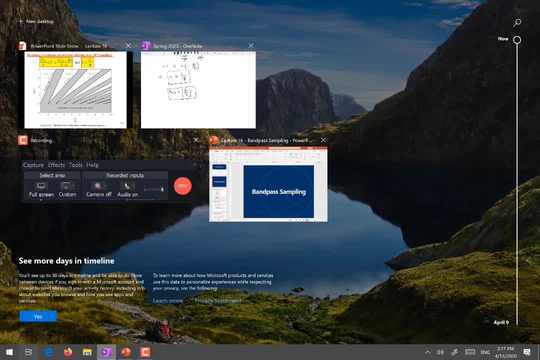 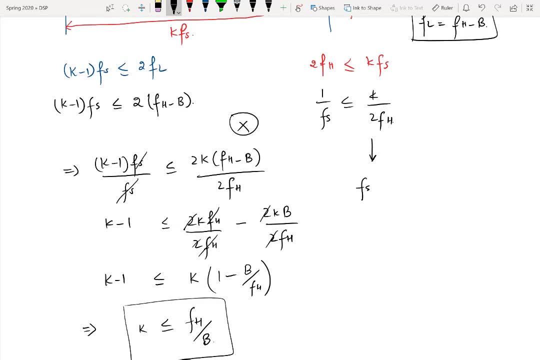 This condition can also be found out by using these two inequalities. So you see, if we are here and you can say from this inequality, you can say that Fs must be greater than or equal to 2 FH over K. So this is the first one. 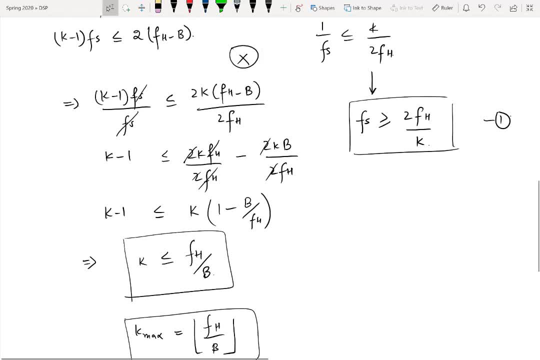 This is the first equation And from this inequality, if I take it over here, you can find out: Fs less than or equal to 2 times FH minus B divided by K minus 1.. So by using these two inequalities, rather by joining these two inequalities, you can end up with the same inequality that we have shown in the previous example. 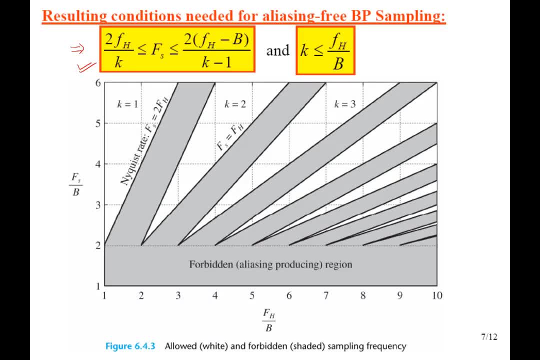 In the slide. this is right. So what does it mean? It means that whenever you are going to perform bandpass sampling and in order to avoid aliasing, you have to select two variables. The first one is K and the second one is Fs. 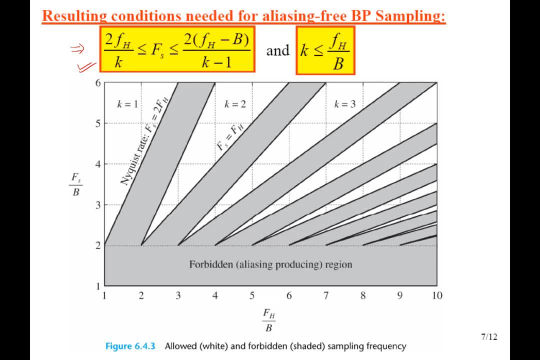 Right. And if you plot all these inequalities and formulate a region so that you can directly find out the sampling frequency, that will avoid aliasing Right. So this results in a very famous plot that is available whenever we talk about bandpass sampling. 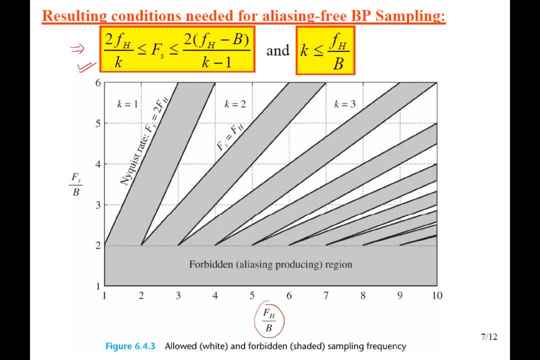 And this plot has two axes. On the x-axis we plot FH over B And on the y-axis we plot Fs over B. It has got multiple straight lines and two kinds of regions. The gray regions are called forbidden regions. It means they are the regions where aliasing occurs. 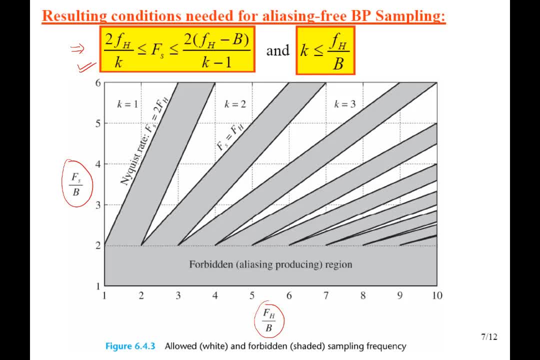 And the white regions are aliasing free regions. So whenever you are going to select sampling frequency, you need to either use the inequalities- these two yellow indicated inequalities- or, if you have this graph in hand, then it is recommended that instead of using inequalities, 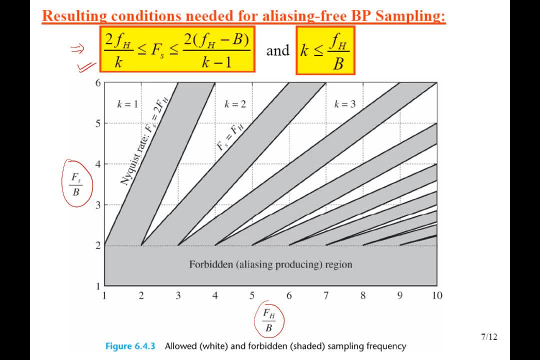 you straight away go to this plot and directly find out the sampling frequency. Now, how to find out the sampling frequency? by using this plot which results in aliasing free bandpass sampling. The procedure is very simple: You first of all find out FH. 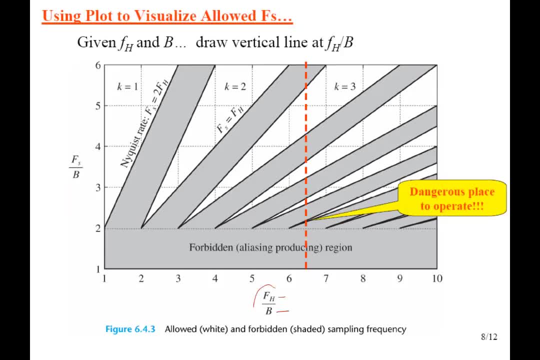 You first of all find out the value of FH and B And you find the ratio. For example, the ratio comes out to be 6.5 in some particular case. So at 6.5, you will draw a vertical line, as shown as a dotted red line, over here. 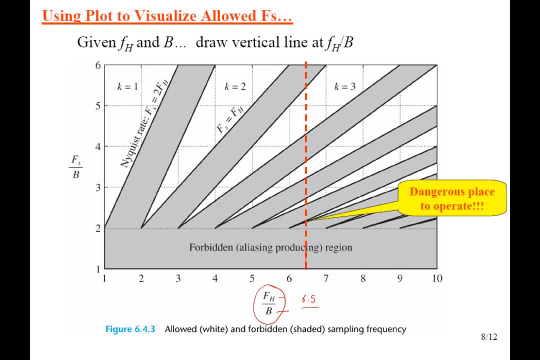 And then for a specific value of K, you will draw a horizontal line. Now, what must be the value of K? Because the second condition was that K must be less than FH over B, And FH over B is 6.5.. 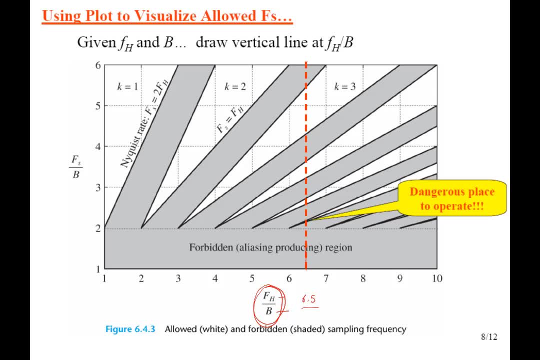 So you can select any value less than 6.5.. But at most you can select K is equal to 6.. Now if you select K is equal to 6, what will happen? Like here: K is equal to 3.. 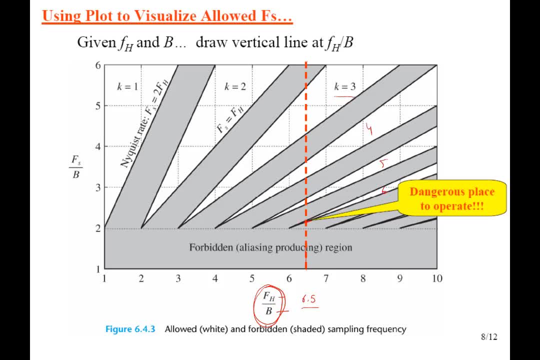 This is 4.. This is 5. And this is 6.. So if you select this region, it is very dangerous to operate because, just as a result of a small error, you can just fall into the category of forbidden region. So you will try to avoid these regions. 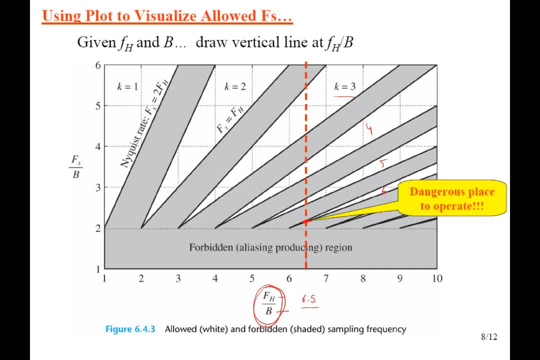 Instead, you will go to lower values of K, So you will prefer to use K is equal to 4 or K is equal to 3.. And, for example, if we operate at, K is equal to 3, it is a normal practice and it is recommended that you select. 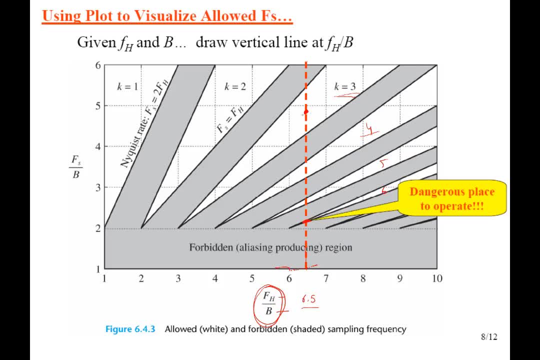 the middle point over here. So you select the middle point and then draw a horizontal line and see where it is intersecting with the y-axis. For example, it is intersecting at 4.7.. So it means FH over B is equal to 4.7.. 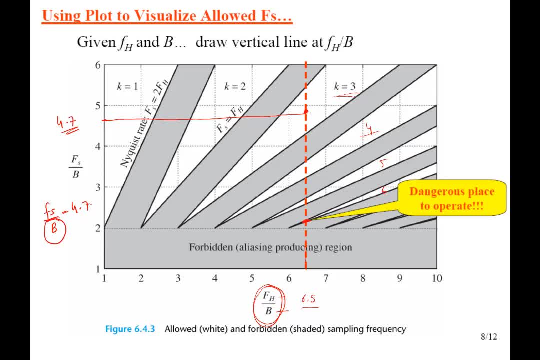 And because you have the value of B, you simply multiply it with 4.7 to get the final sampling rate at which you need to sample in order to avoid the aliasing. You see, the selection of K is in your hand And you have to avoid aliasing.